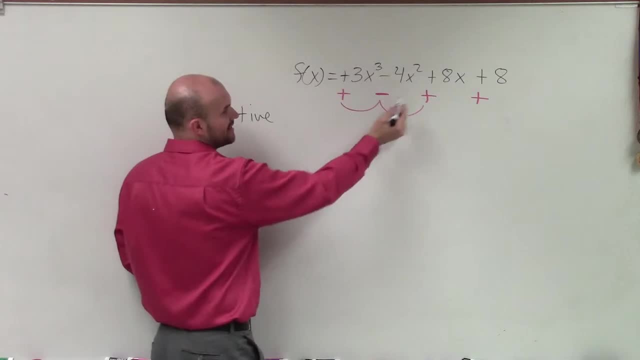 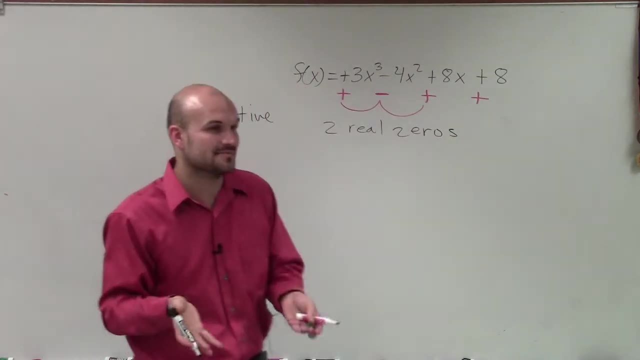 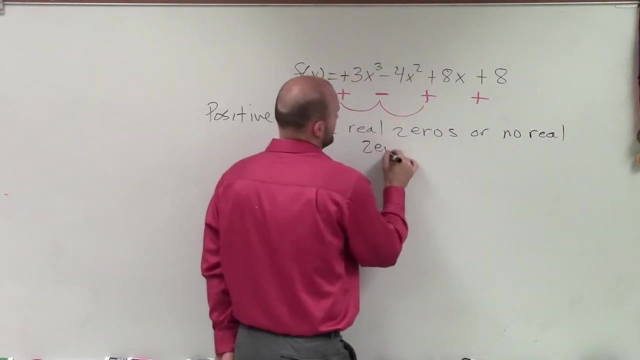 we have. So we've had two alternating signs, from positive, negative, negative positive. Therefore, there's two real zeros, but that's not it. There's a possibility of having two real zeros or no real zeros. 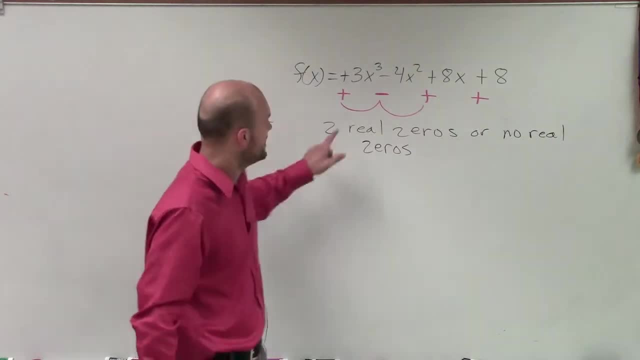 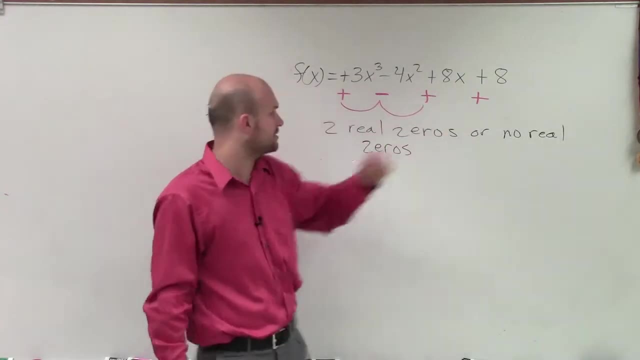 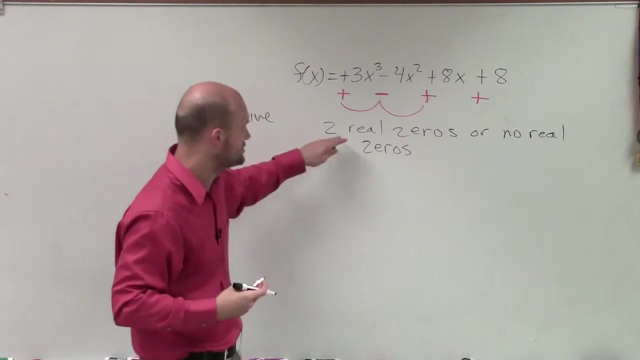 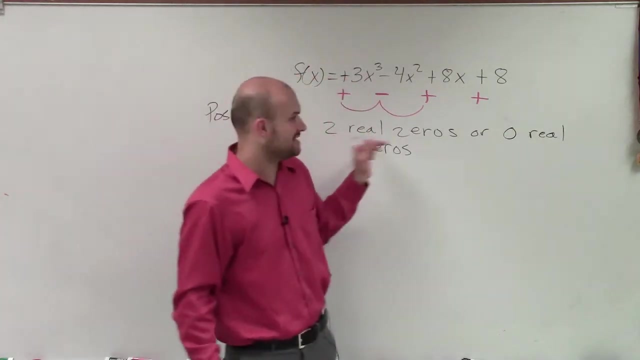 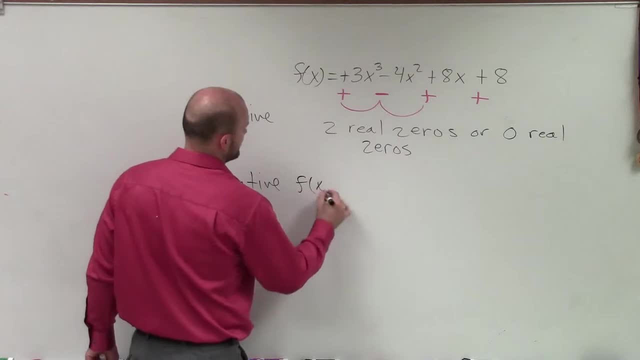 So to look at the negative real zeros again, you just do f of x. But now, instead of writing the f of x for the positive, we're now going to evaluate for negative f of x. So now what I do is I have 3 times negative x cubed. 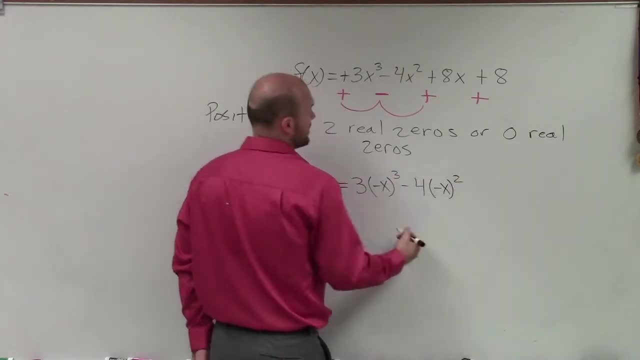 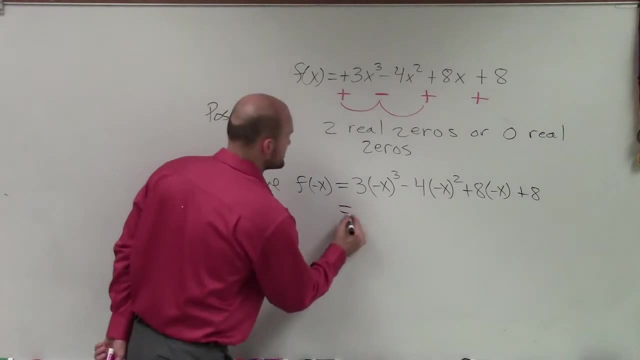 minus 4 times negative x squared plus 8 times negative x plus 8.. So now we go ahead and simplify this. Well, any negative number- it doesn't matter, you know, it's an x- Any negative number raised to the third power. 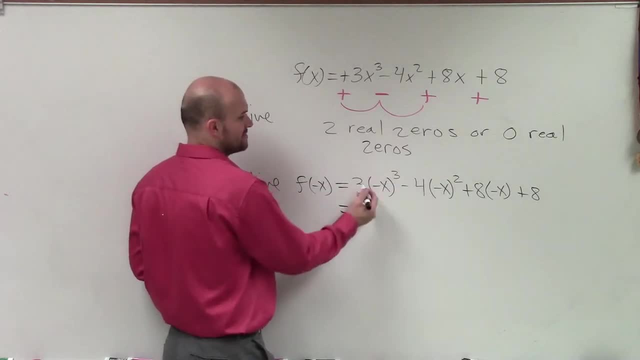 is still going to be its sign. So a negative x cubed times 3 will now be turned to a negative x cubed. Anything negative squared is going to be positive. Positive x squared times negative will be a negative 4x squared. 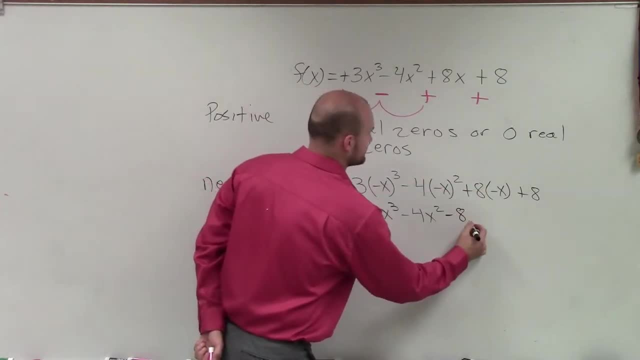 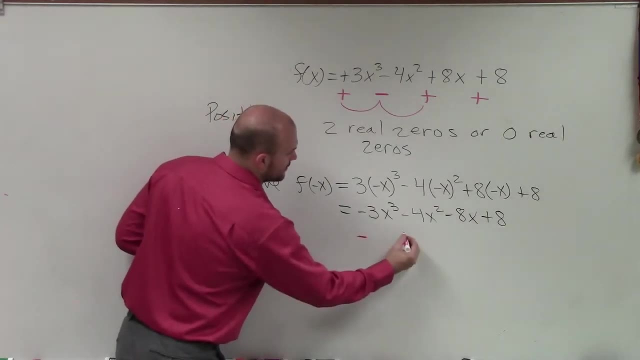 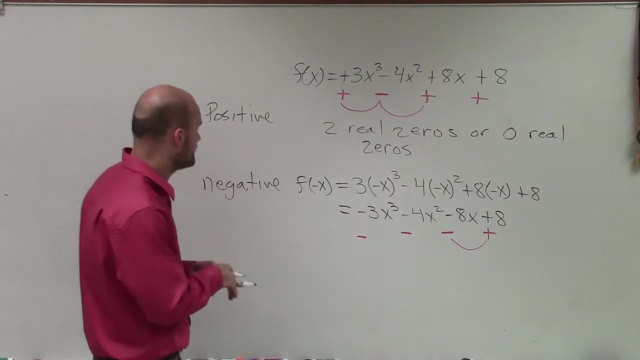 Negative x times 8 will be a negative 8x And then plus 8.. So again, let's bring down the signs: Negative, negative, negative, positive. So now you can see There's one interchange. So the number of negative possible real 0s. 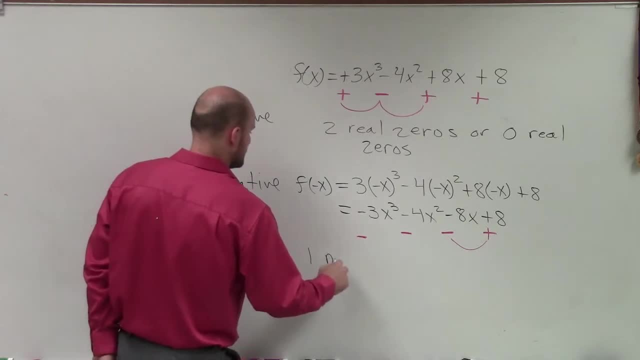 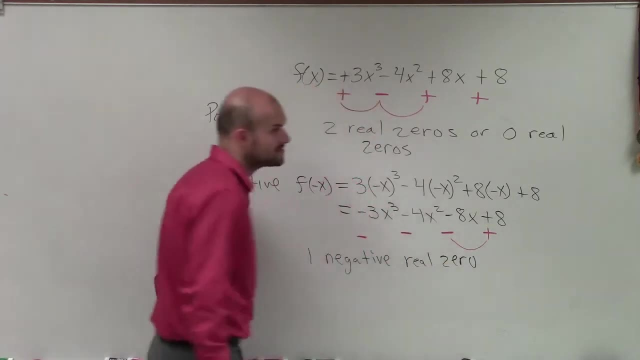 or the number of negative 0s is now going to be 1 negative real 0.. Now the problem is, we can't subtract. You say, well, this one, you subtracted 2, right, You subtract an even number.